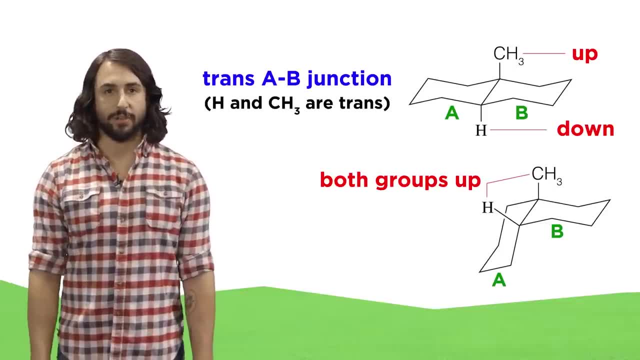 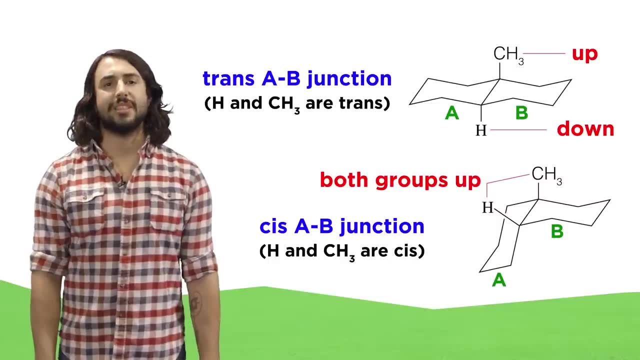 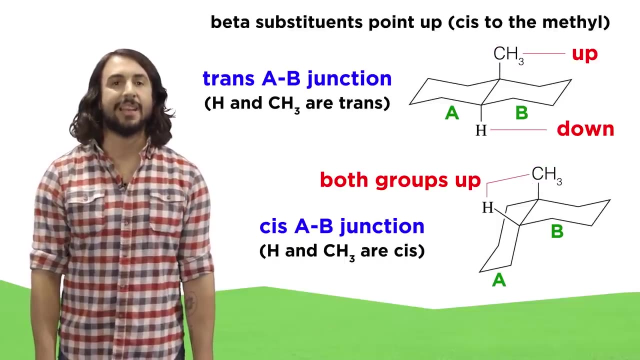 for the A ring, either with a trans-ring junction between A and B like this, or a cis-junction putting ring A like this. Also notice that the methyls are in the axial position pointing upwards, and we will commonly refer to the substituents on the same side. 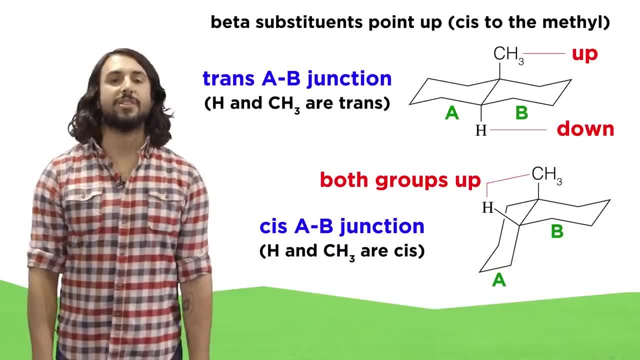 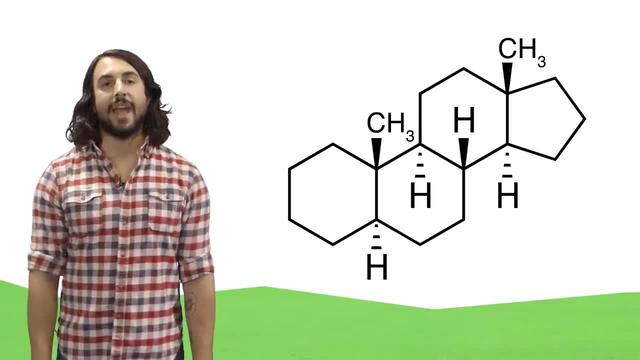 as those methyls as beta substituents, whereas ones on the other side trans to the methyls, will be alpha substituents. The orientation of the A ring will depend on the hydrogen at carbon five. If that hydrogen is alpha, or on the dash bond, you get the trans-ABD. 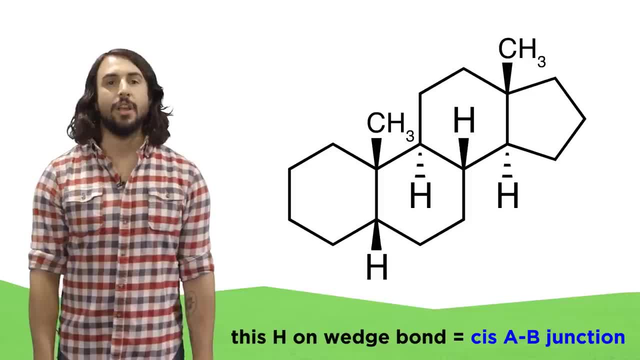 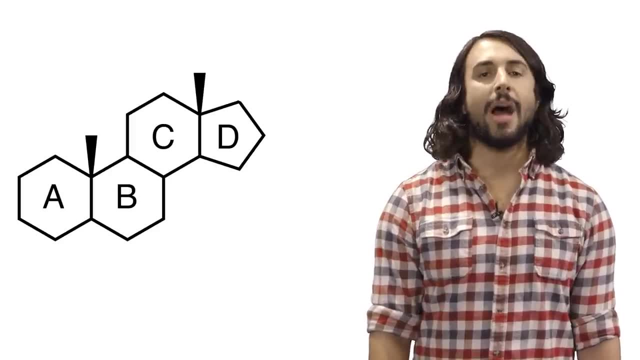 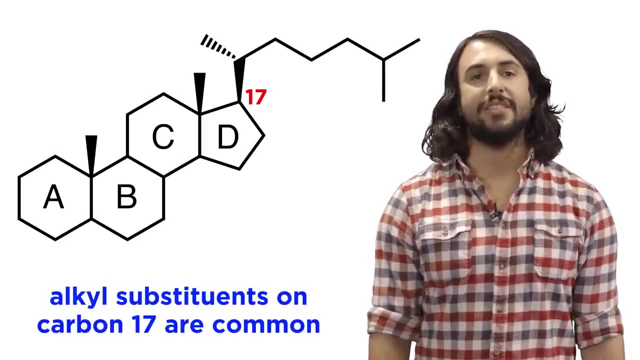 If the hydrogen is beta or on the wedge bond, you get the cis-ABD. Now, where else do steroids vary in structure? A common location for a substituent is carbon 17.. Different alkyl groups at this location will generate different steroids, one of which 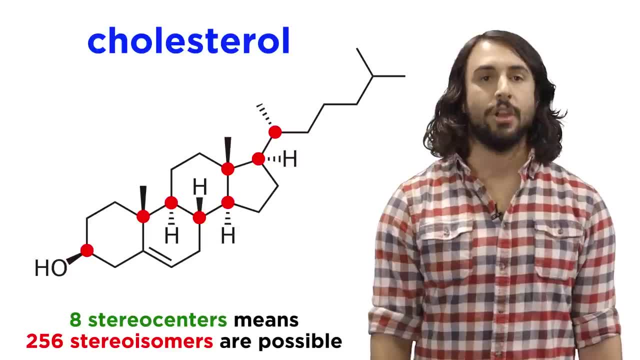 is cholesterol. Cholesterol has eight stereocenters, which means 256 different stereoisomers of this structure are possible, but only this specific structure is possible. That means that the number of different stereoisomers is not the same as a substituent. 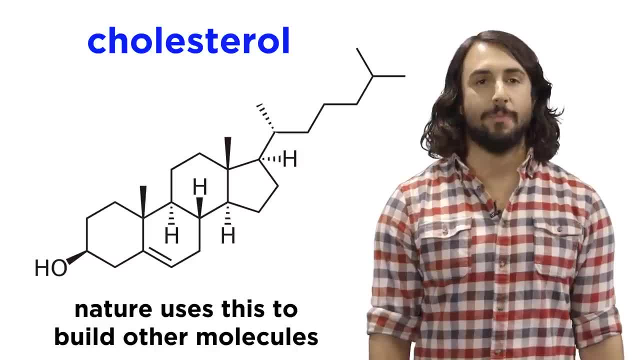 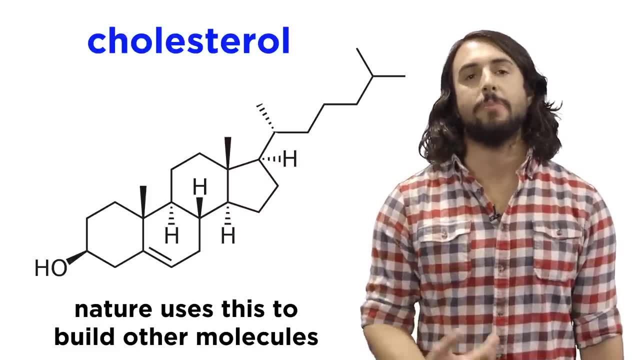 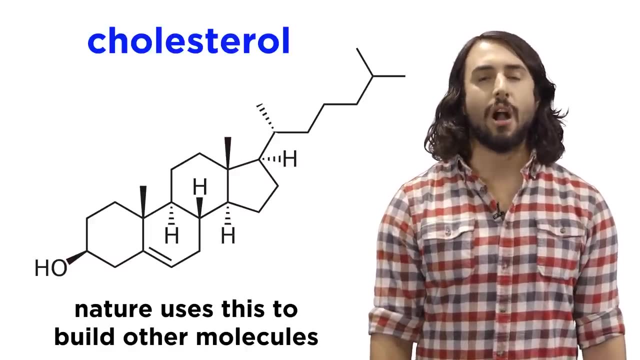 specific one is cholesterol. this is an intermediate in the biosynthesis of all the steroids we need in our body, and although we often consume cholesterol, we don't need to because we also make it ourselves. so we will typically have more cholesterol than we need, and too much cholesterol in the diet leads to clogged. 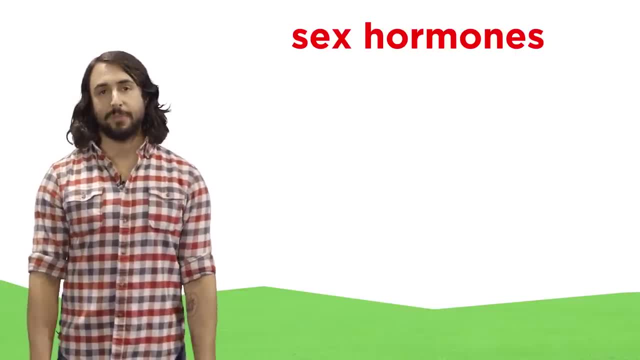 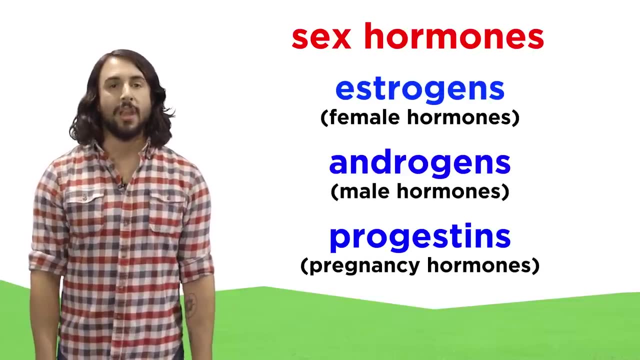 arteries and heart problems. let's look at another type of steroid: the sex hormones. these can be divided into three classes: the female hormones, or estrogens. the male hormones, or androgens. and pregnancy hormones, or progestins. let's 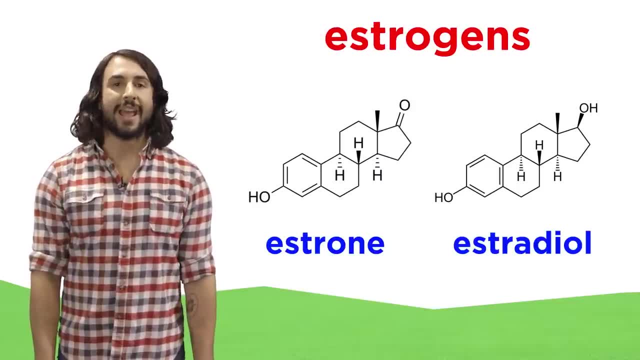 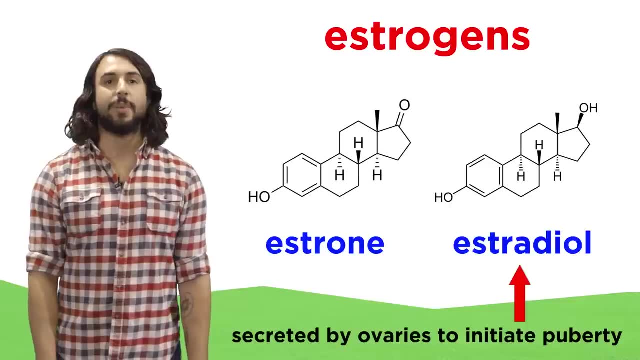 look at the female hormones first. these are estrone and estradiol, which differ only in the level of oxidation at carbon-17.. estradiol is secreted by the ovaries and kicks off the changes that occur during puberty and also causes 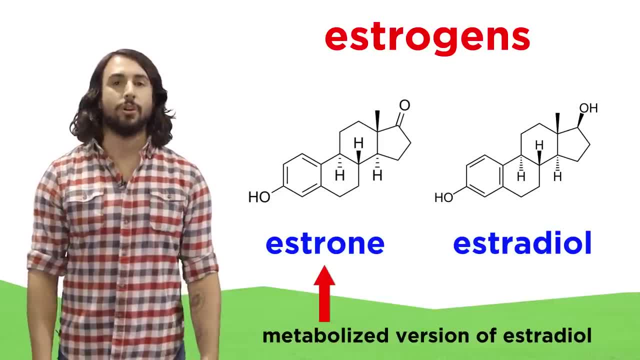 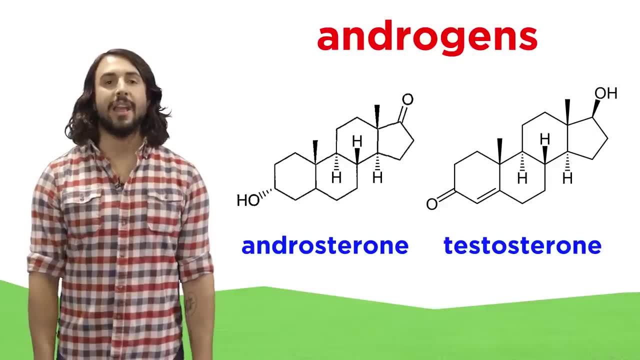 development of the mammary glands during pregnancy, whereas estrone is just a metabolized form of estradiol that is excreted, the male sex hormones, androsterone and testosterone, are incredibly similar to the female hormones, with the only differences occurring in the A-ring.